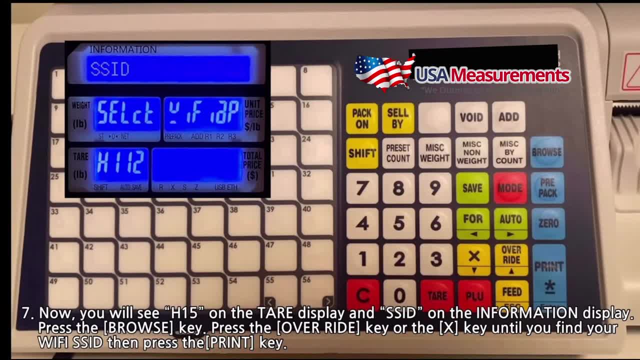 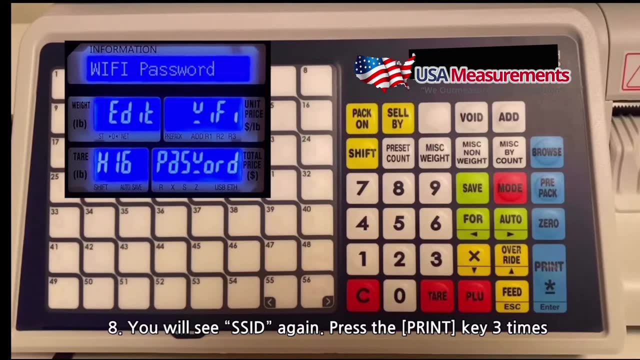 Now you will see H15 on the tear display and SSID on the information display. Press the browse key, Press the override key or the X key until you find your Wi-Fi SSID. then press the print key. You will see SSID again. Press the print key 3 times. 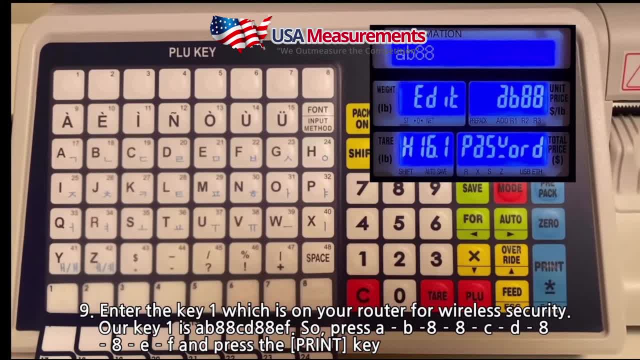 Enter the key 1, which is on your router for wireless security. Our key 1 is AB88cd88ef, so press AB88cd88ef, then press the print key. Just to make sure if the H17 OFF Mode is 0, which means it's opened, press the print key. 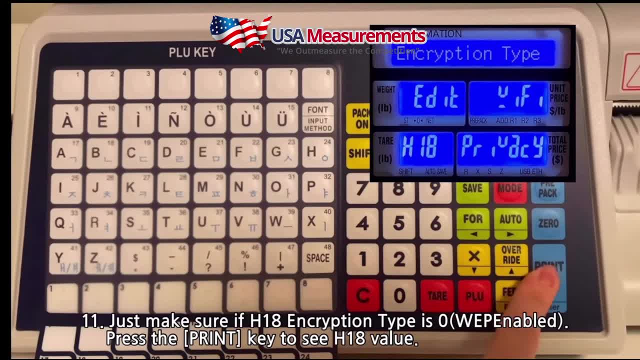 to see the H17 value. Just make sure. if the H17 O Emirates Value or the H17 Hey beer value are boxed will be available. This means that the H17 H1 also connects to your PC to your H18. encryption type is 0.. Press the print key to see the H18 value. 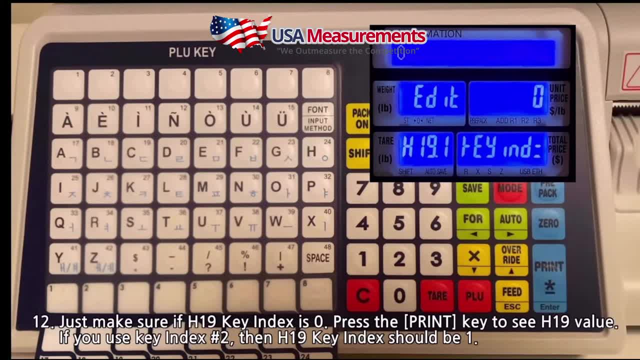 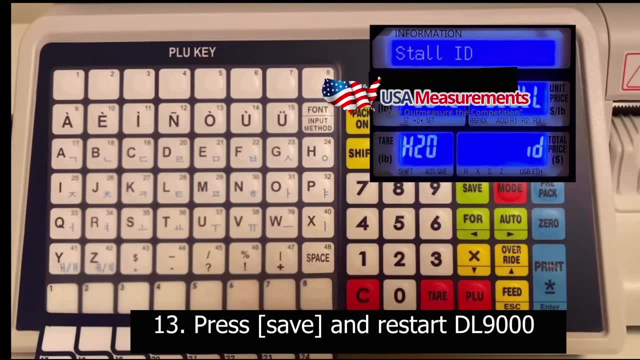 Also make sure that the H19 key index is 0.. Press the print key to see the H19 value. If you use key index 2, then H19 key index should be 1.. Press save and restart the DLP 300 scale. First of all, if you want to find your PC IP address and the DNS server's IP address, go to Internet Access, then Properties. You will see your PC IP address, DNS server's IP address, Wi-Fi SSID and etc. 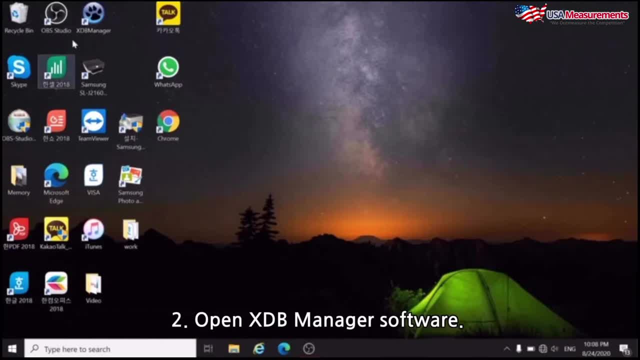 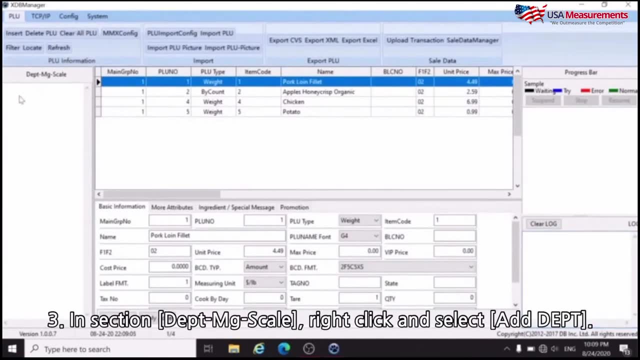 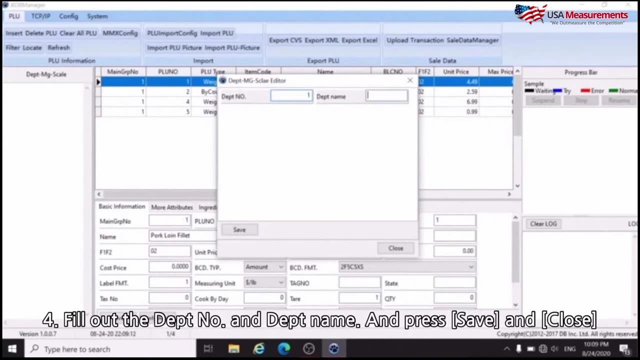 Open the XDB Manager software. In section Department MG Scale, right-click and select Add Department. Fill out the department number and department name, then press save and close. In section Department MG Scale, right-click and select Add Department. In section Department MG Scale, right-click and select Add Department. 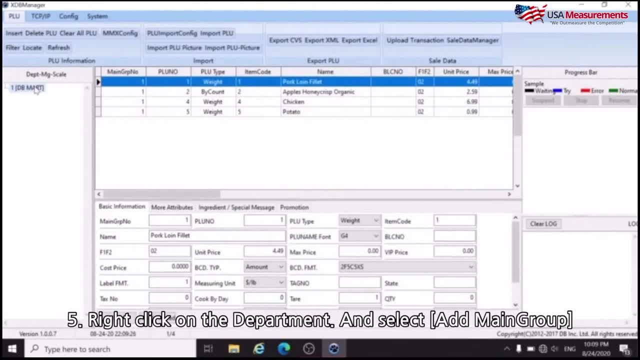 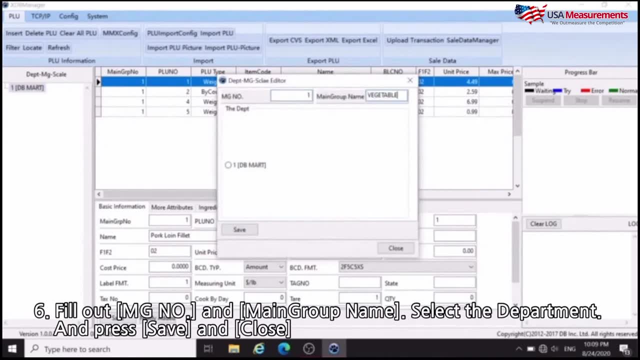 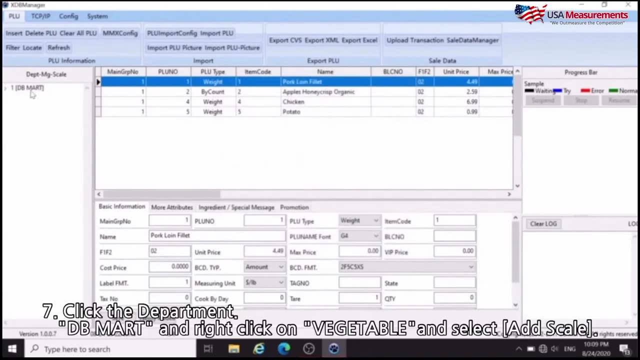 Right-click on the department and select Add Main Group. Fill out the main group number, the main group name. select the department, then press save and close. Click the department- In this example it's DBMark. Right-click on Vegetable and. 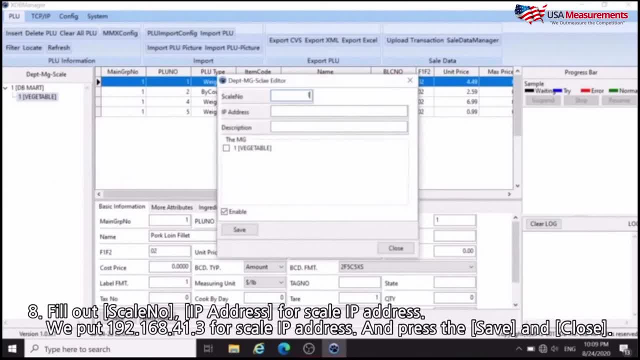 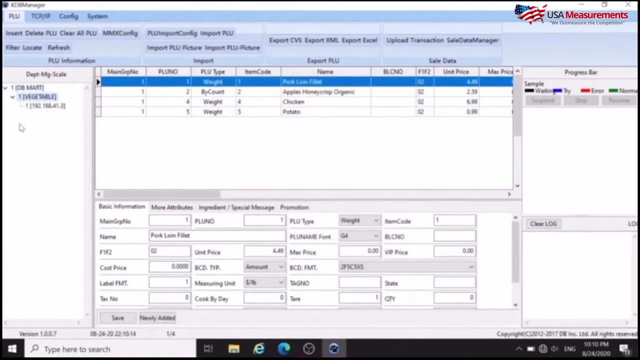 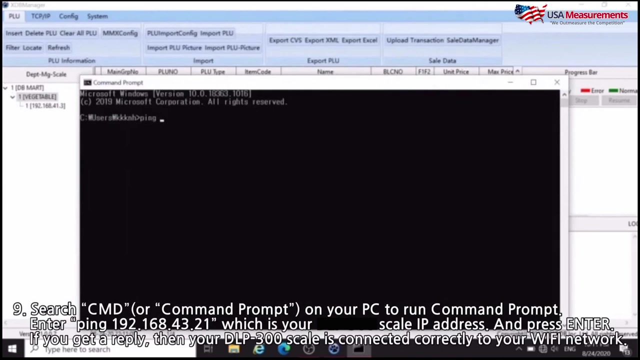 select Add Scale. Fill out the scale number and select Add Scale. Click the department number and IP address. for the scale IP address We put 192.168.413 for our scale IP address. Press save and close. Search CMD or Command Prompt on your PC to run Command Prompt. Enter ping 192.168.4321,.